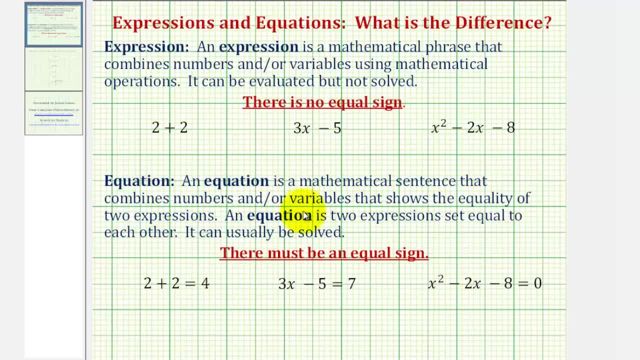 An equation is a mathematical sentence that combines numbers and or variables. that shows the equality of two expressions. So the key here is: an equation shows equality and therefore an equation is two expressions set equal to each other, and normally we can solve equations. 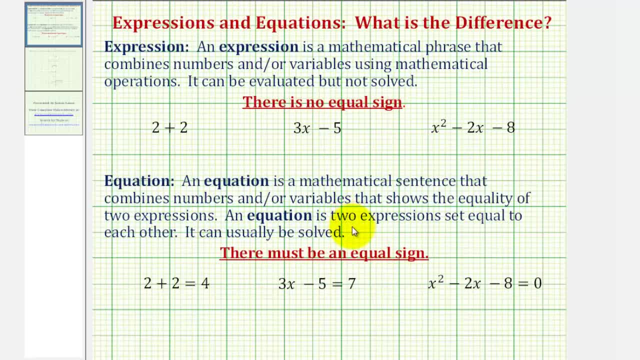 but sometimes equations don't have. So we're going to look at an equation. So an equation is a mathematical sentence that combines numbers and or variables, but sometimes equations do not contain equal signs. But the key to remember here is that because an equation expresses equality, 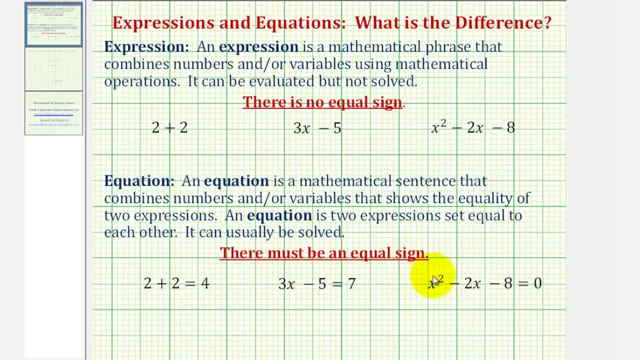 all equations must contain equal signs. Looking at our three examples, notice how all three of them contain equal signs, showing two expressions equal to each other. So before we look at these solutions to these equations, let's go back up to our expressions Again. we already said that we know that two plus two is equal to four. 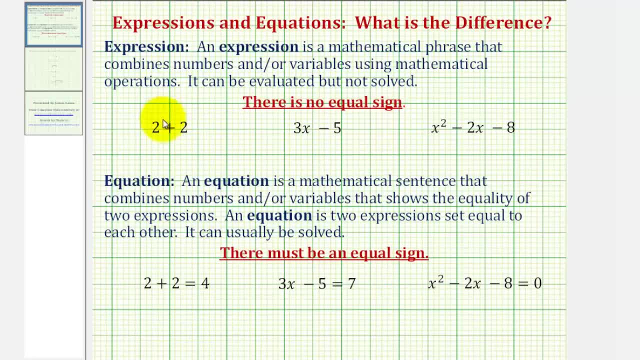 and therefore we can write an equation to show the value of this expression. I think this is where some of the confusion comes into play Again. we know that two plus two equals four, so we just wrote an equation to show the value of the expression two plus two. 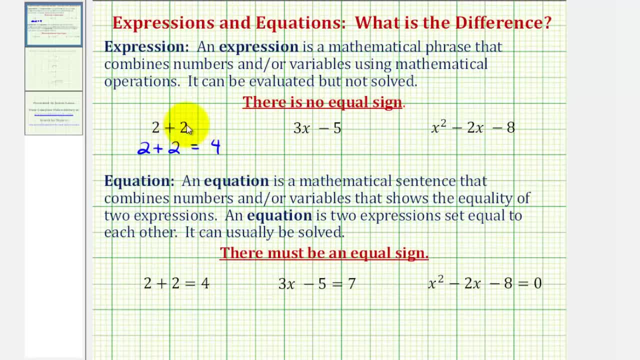 But again we were given an expression, not an equation. For the expression three x minus five, let's say we were given x equals ten. Well, if we're given a value of x, we can evaluate this expression. in this case, 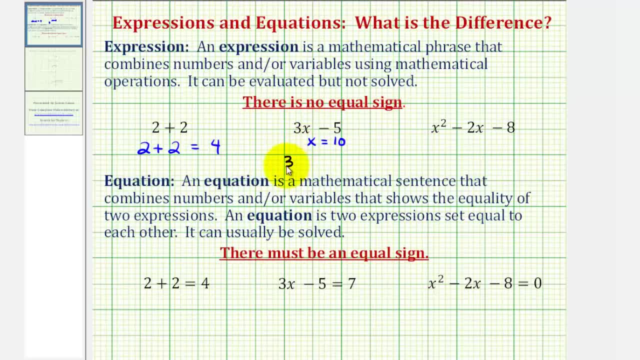 by substituting ten for x. That would be three times x minus ten, instead of three times x minus five. This would be 30 minus five or 25.. Again, notice how we just wrote an equation to show that the expression is equal to 25. 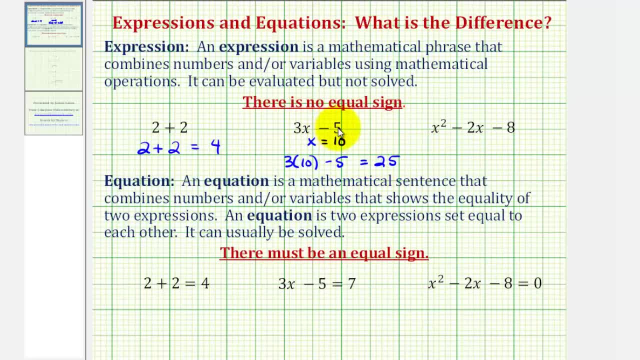 when x equals ten. But again, we were given an expression, not an equation. So this is not a solution. This is just the value of the expression when x is ten. For our third expression, let's say we were given x equals five. 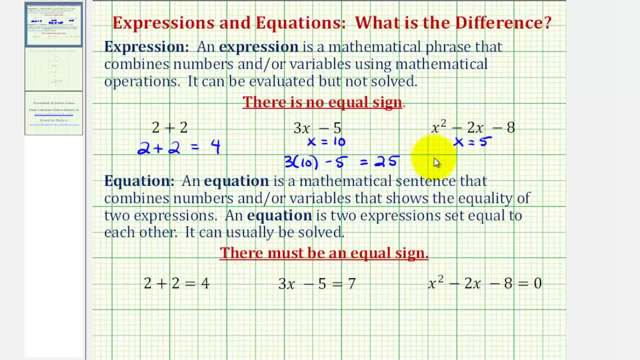 So this is not a solution. This is just a given value of x, So we'll substitute five for x to evaluate the expression. Well, this would be 25 minus ten, That's 15 minus eight, which is equal to seven. 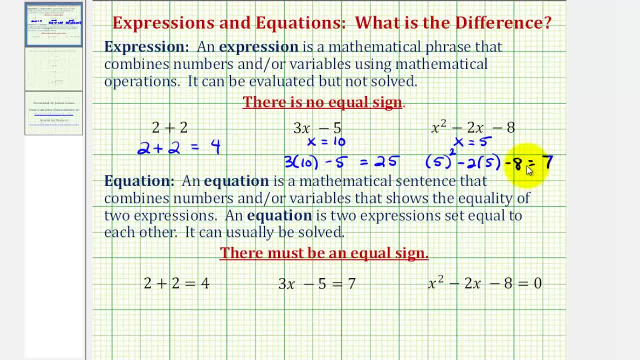 Again. we just wrote an equation to show the value of the expression when x equals five. Now let's go back down and look at our equations. Two plus two equals four is an equation, even though it doesn't contain a variable. notice how this equation is always true and therefore 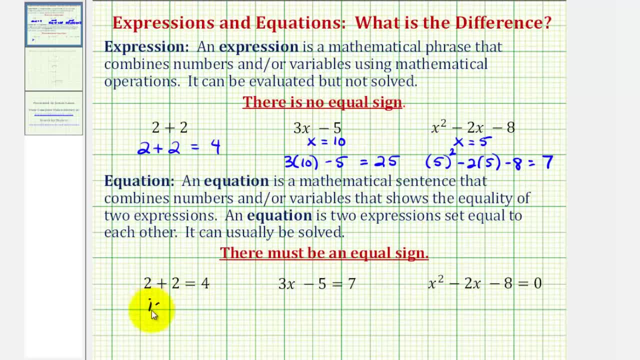 it has a special name, that's called an identity. Next, the equation three x minus five equals seven has a solution. The solution is x equals four. The reason it's a solution is that when x equals four, the expression on the left is equal. 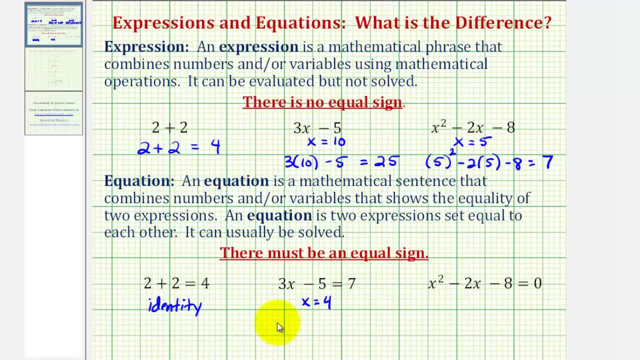 to the expression on the right, or if we substitute four for x, we would have three times four minus five equals seven. Well, this would be 12 minus five, which is seven. Seven equals seven verifies x equals four is our solution. 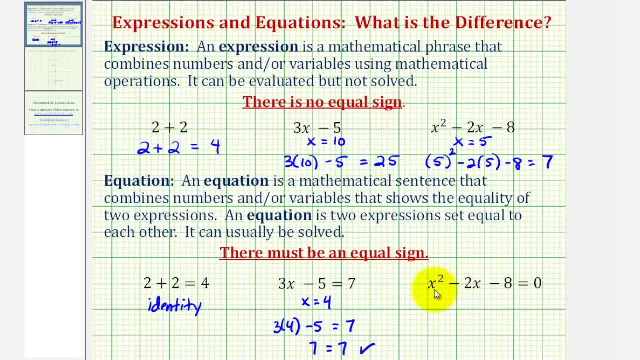 And for our last equation, because of the x squared, we actually have two solutions. One solution is x equals four and the other solution is x equals negative two, which means if we substitute four for x or negative two for x- the expression on the left- 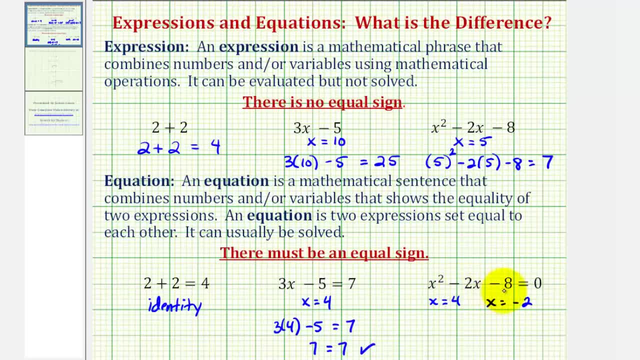 will equal the expression on the right or the left side will equal zero. Let's go ahead and verify that. If x is four, we would have four squared minus two times four minus eight equals zero. Well, this would be 16 minus eight minus eight, which does equal zero. so that's true. 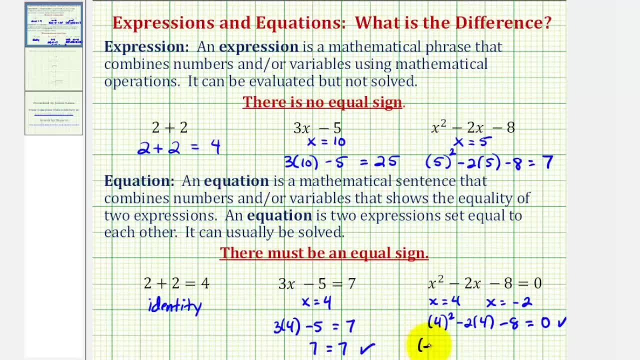 X equals four is a solution. and then when x equals negative two, we would have negative two squared minus two times negative two minus eight equals zero. We'd have four plus four minus eight, which does equal zero, verifying our solutions. So, again, the main thing to remember is: an expression does not contain an equal sign. 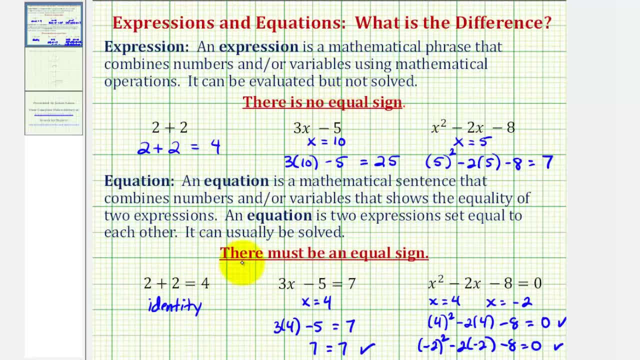 therefore it can't be solved, but it can be evaluated and an equation must contain an equal sign and, in many cases, can be solved. I'll just emphasize this one more time to determine which of these are expressions and which are equations. 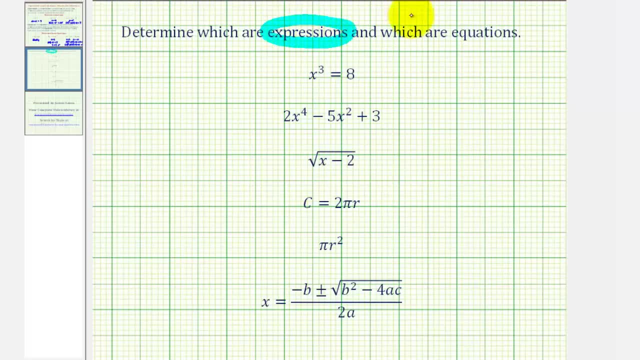 Let's go ahead. Let's go ahead and circle the expressions and put boxes around the equations. First we have x cubed equals eight. We have an equal sign and therefore we have an equation. Next, we have two x to the fourth minus five, x squared plus three: no equal sign.